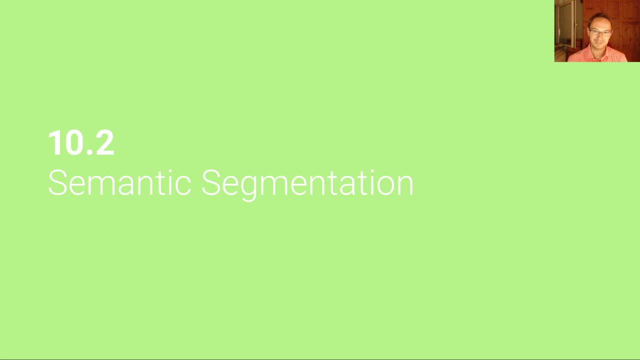 Now let's move on to semantic segmentation. There have been a few attempts to semantic segmentation, also before the deep learning era, but the performance of these approaches is nowhere near comparable to the performance of deep methods, so we're going to focus on deep methods in this. 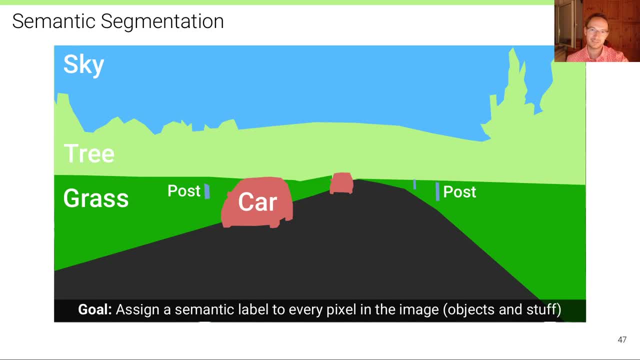 unit. Let's remind ourselves again what is the problem. The problem is given an input image that is not shown here, but you can imagine what it looks like- to classify or assign a semantic label to every pixel in that image. So, for example, 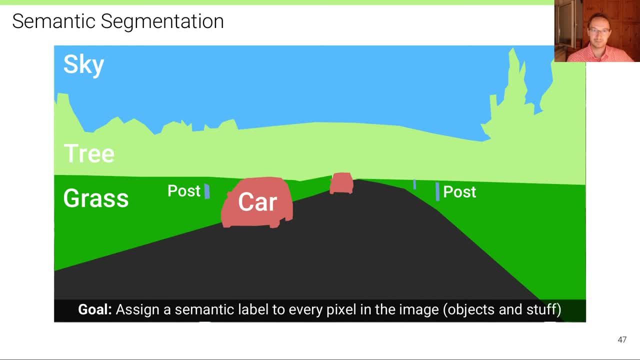 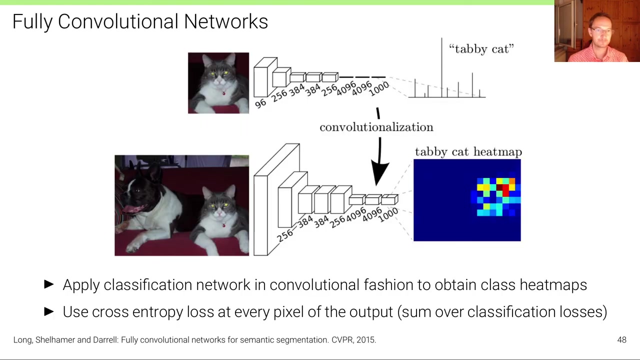 this pixel here we want to associate with the class sky, which might be label number 5.. And this pixel here we want to associate with the of the label grass, which might be pixel number 13 and so on. this is the goal and we want to do this for both objects like cars and stuff categories like sky in. 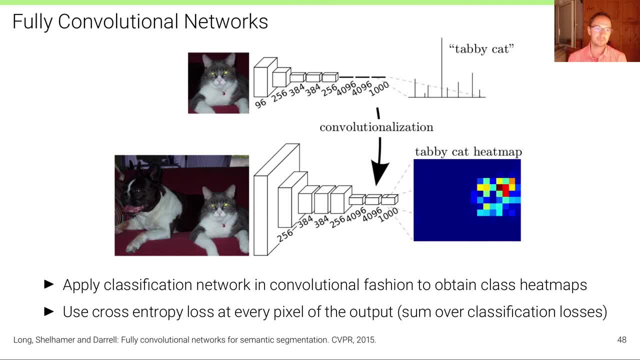 2015, a group at Berkeley realized that actually we we can obtain semantic segmentation using a classification network. they observed that, given that the the very strong performance of image classification networks, why can't we just apply those classification networks in a convolutional manner on larger images and instead of producing a one by one output which is turned into a? 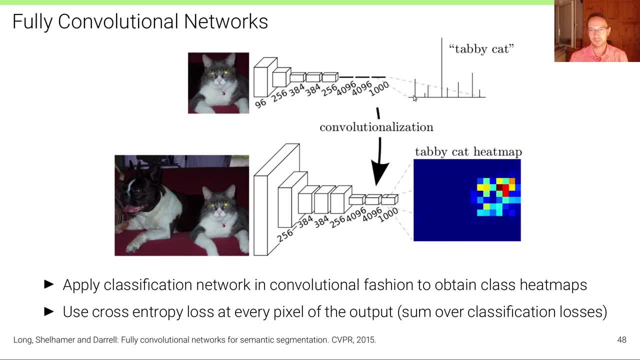 probability distribution, as we have seen in the previous slides, return a feature map that is converted into several heat maps, one heat map per category. here is the heat map for tabby cat and, as you can see, now, in addition to the classification results we have some red pixels that indicate strong. 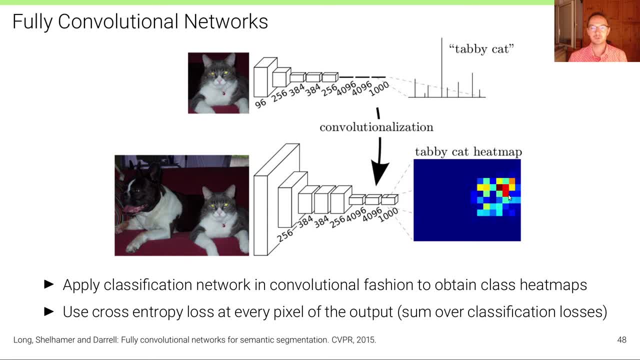 probability for the presence of tabby cat and, as you can see, now, in addition to the classification results, we have some red pixels that indicate strong probability for the presence of tabby cat. we also know where the presence of this class is, because we have applied this. 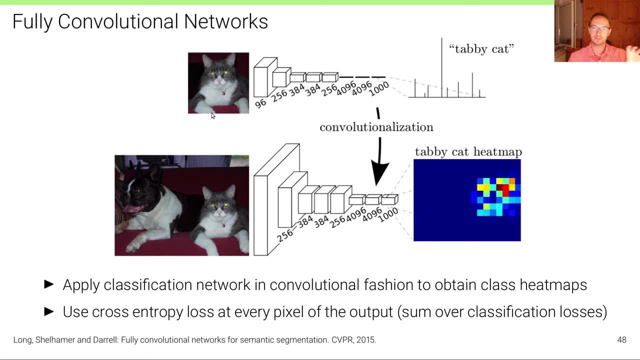 network here in a convolutional manner, in a sliding window manner over this image, but of course we have implemented it as a big convolutional network and so we have this heat map here that tells us for the category tabby cat where there is high probability for that category. so we apply this heat map here and we can see that the 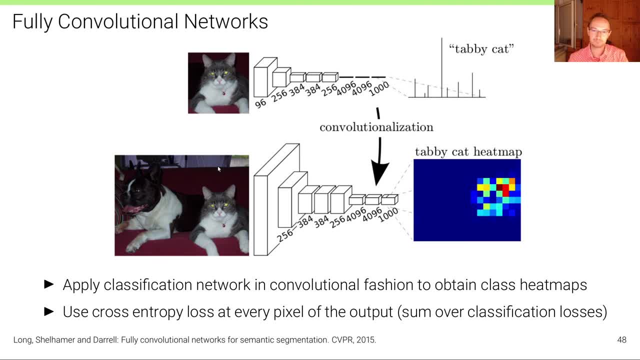 generalization will be high in case of middle class. in the cohesive example, original code for class, complete and also ultimate, and then we can use such a nuts function for class. Well, look at thisや what the new? uh same as a classification network, except that now we have a sum over losses where 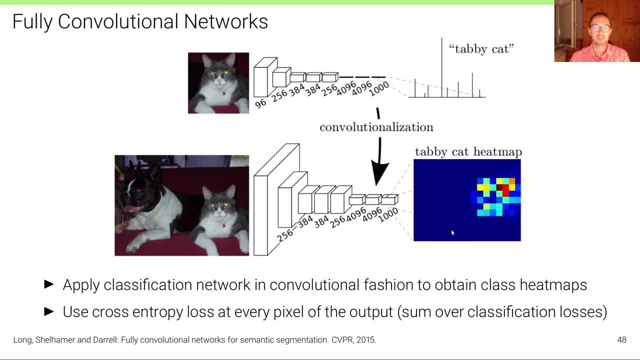 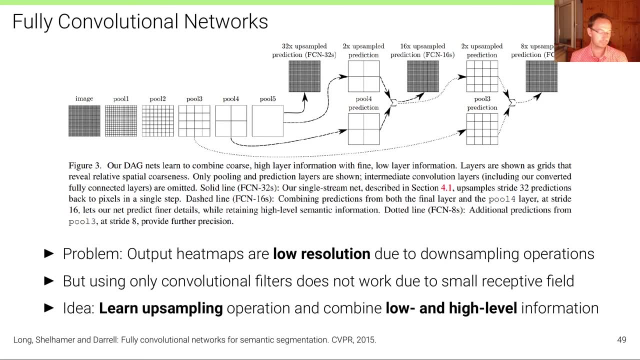 we have one classification loss for each of these pixels in this stack of heat maps. however, the problem, as we can already see from here, is that the output heat maps are really low resolution due to all the downsampling that takes place in the neural network in order to achieve a large receptive field, that is. 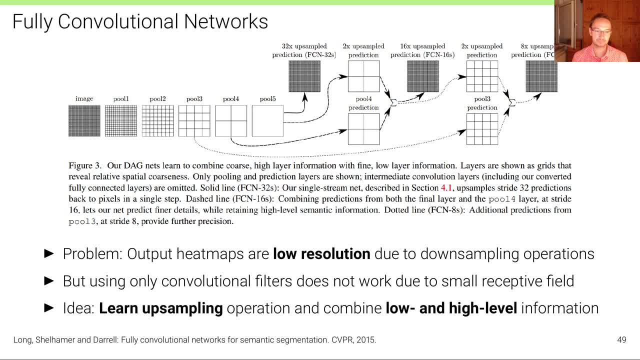 necessary in order to actually recognize the object. however, using only convolutional filters without any down sampling does not work in practice due to the small receptive field. in other words, I would need a huge amount of convolutional filters, hundreds of layers, in order to obtain the same large 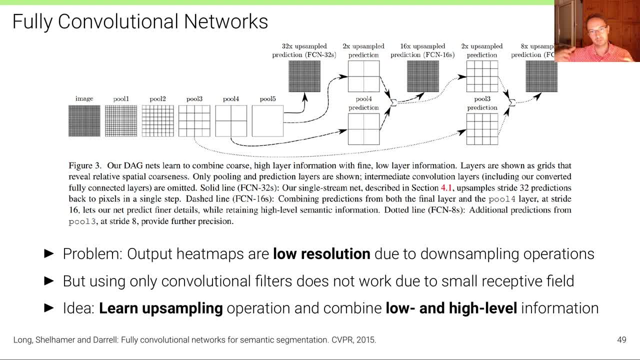 receptive field that I can obtain with just a few down sampling operations, such as max pooling, and this is just impossible to train. the number of parameters is too large and this is just impossible to train. the number of parameters is too large and this is just impossible to train. the number of parameters is too large. 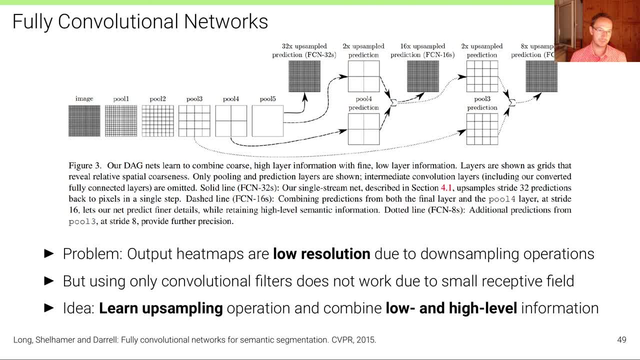 this doesn't work. the idea, therefore, in this paper- and it's something that has maybe gone a little bit unnoticed, but a lot of the ideas that are present in modern semantic and instant segmentation networks are already present in this original paper from 2015. this core idea, the second core idea, apart from the 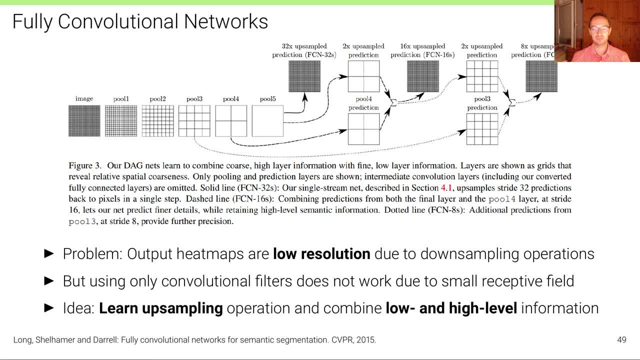 convolutional ization is to learn also an up sampling operation and combine low and high level information. so here you can see, indicated by this grid structure, the resolution that we're operating on. here's the image. the convolution layers are not shown just for clarity, but there's some convolution layers here than pooling conf, pooling conf pooling. 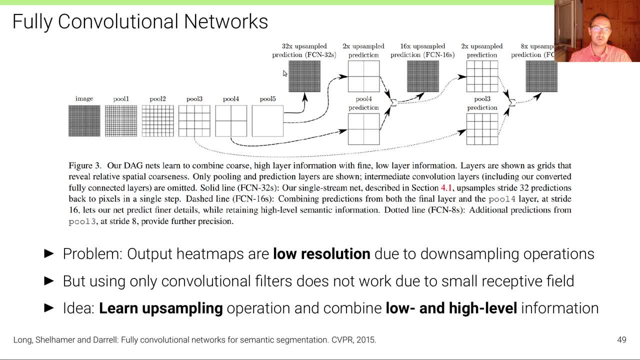 and so on, and then, in the most basic version, here are this: from this very, from this very low-resolution, We directly up sample with one layer of French caping called deconvol�ution is a. This is a cross between the two layers. theög Kotτικ for happened. 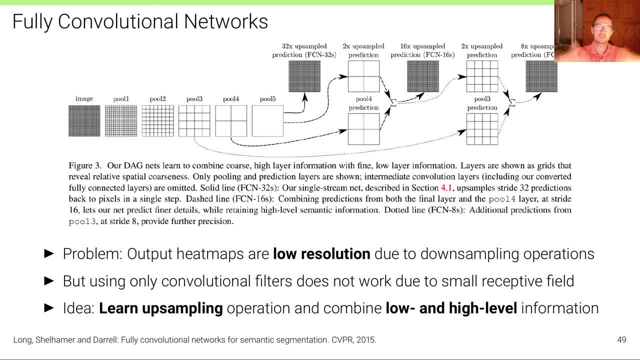 Post convolution. the inverse is, the model is 1iptic inverse of a convolution is an upsampling operation. it's one form of doing upsampling. so here we, upsampling directly from this very coarse resolution to this very fine resolution. of course the model cannot recover the fine details, but what we can do is we can upsample. 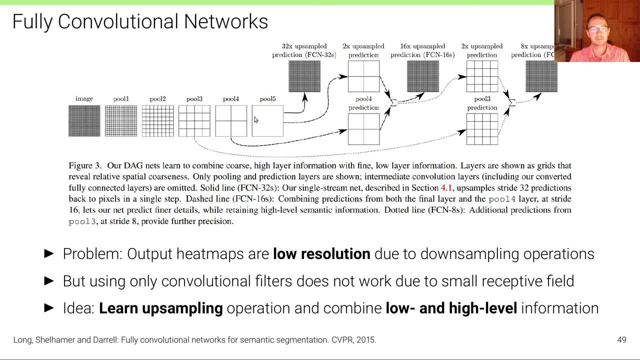 from here to just this resolution, um, like the next one. and then take features from that layer and combine them, add them or concatenate them, and then do the same again: upsampling, the transpose, convolution, the learned, up sampling, and then combine with a sum or concatenation, with 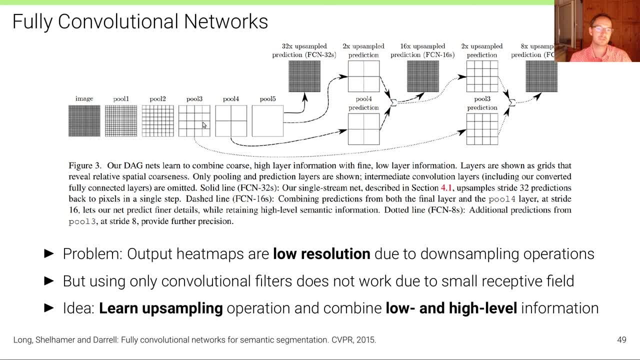 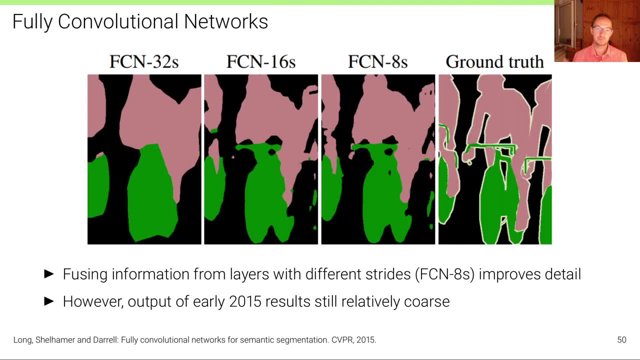 the features at that level and therefore, because these features here already contain some information about the edges, some high frequency local feature information, we get sharper boundaries and this is illustrated here. fusing information from layers with different strides improves detail. here's this very simple variant and here is the variant that fuses these features from the layers with the different strides. 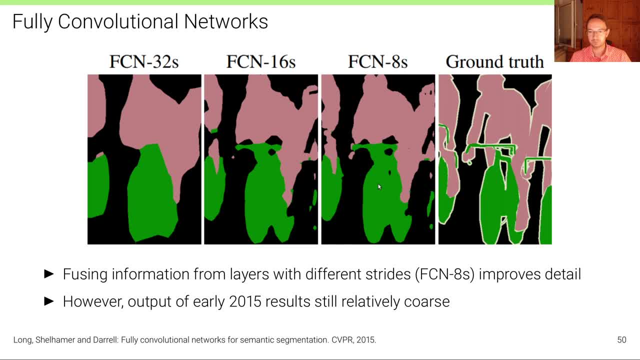 however, as you can still see from these results, even for relatively simple examples, the output is still relatively coarse. this is 2015.. this is the first approach to the problem, still beating all of the state of the art in terms of classical approaches, and then, from there on, of course, the quality improved. 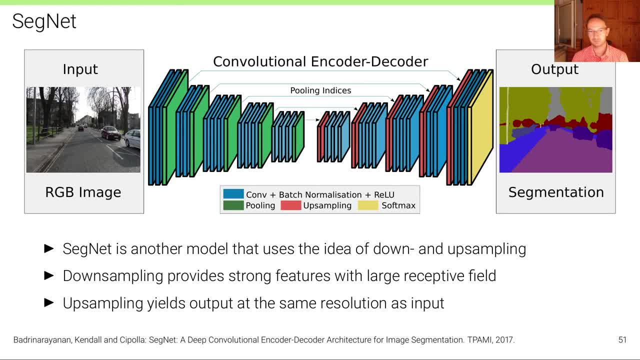 here's another model that has been developed around the same time concurrently. they all have a similar architecture. it's all an encoder. we have this, this part of the network that is contracting, where the spatial dimension is reduced and the feature channel number is increased. and then there, 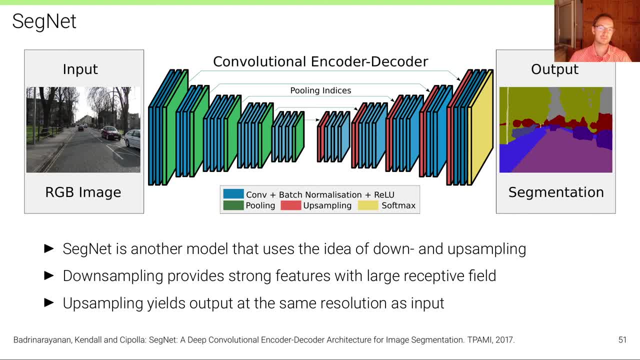 is a, an extension part here on the right where it's called a decoder, where information is decoded back up to the highest resolution, and there's the skip connections. in this case they they skip just the pooling indices in order to retain high detail. so there's a couple of different ways to do the skip connections. 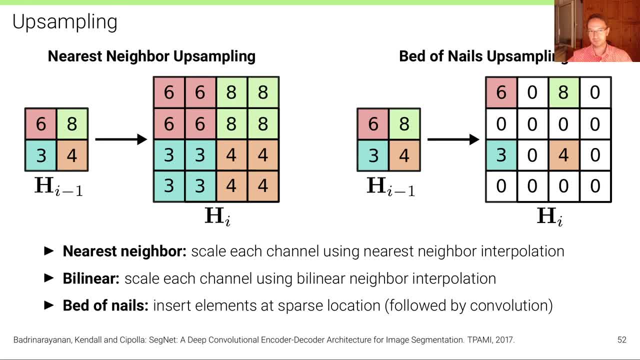 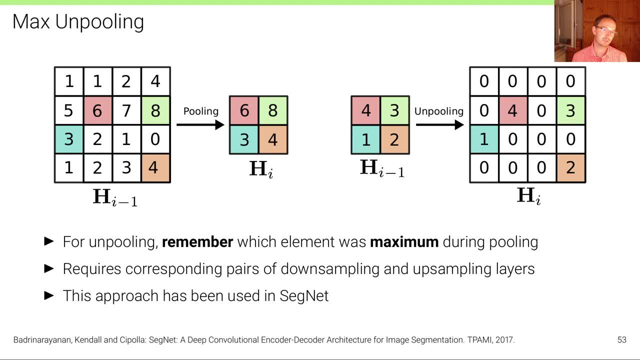 so, for example, like for the up sampling operation, we can do nearest neighbor up sampling or bed of nails upsampling or bilinear sampling. but what they did in this particular sec network is they used these pooling indices that they basically in every pooling operation they remember which. 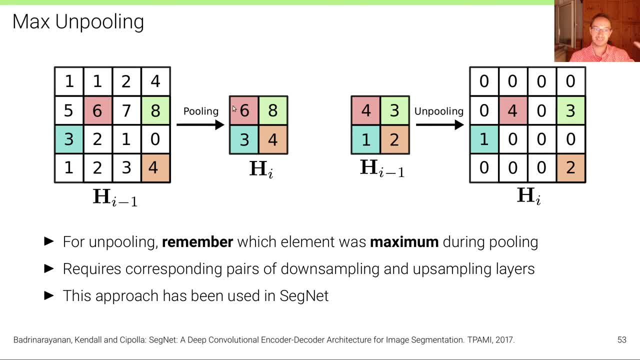 element was activating maximally. it is a max pooling operation. so in this case this element and then in the unpooling operation we injected this information by unpooling into that location. so for example, here the six was most strongly activated, so the four in the respective unpooling. 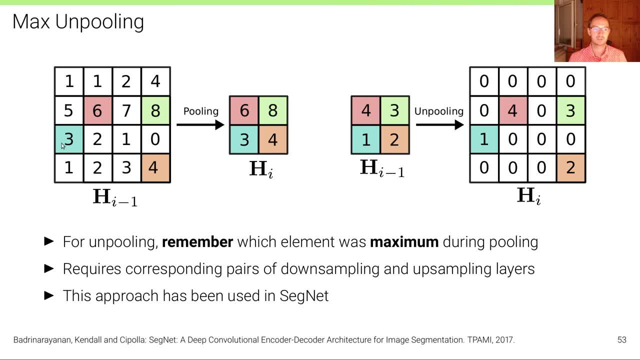 operation gets inserted here. here the three is most active or most most strongly activated, and so the one in the respective at the same resolution. unpooling operation gets inserted at that same location. so, for unpooling, remember which element was the maximum during pooling and this is where the location where the element is. 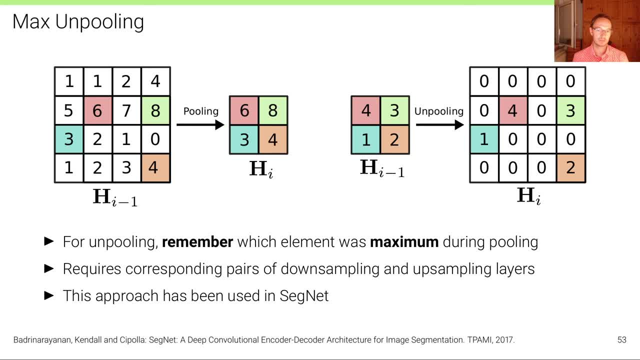 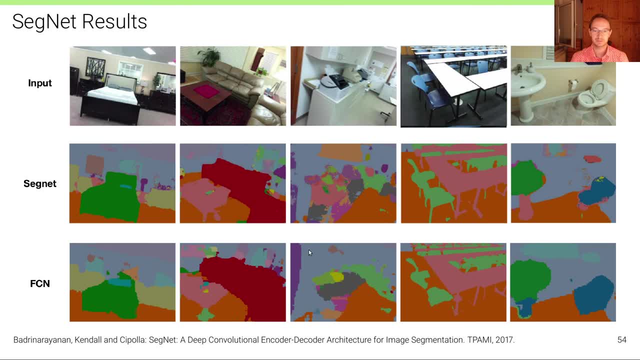 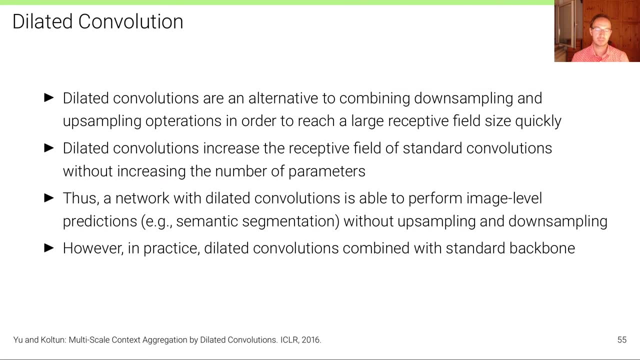 inserted and here's some results of the second model and it compares also to the fully convolutional model and you can see that this particular type of skipping improves results. an alternative to downsampling and upsampling or a model that can be used in combination, actually is a so-called dilated convolutions. they are an alternative. 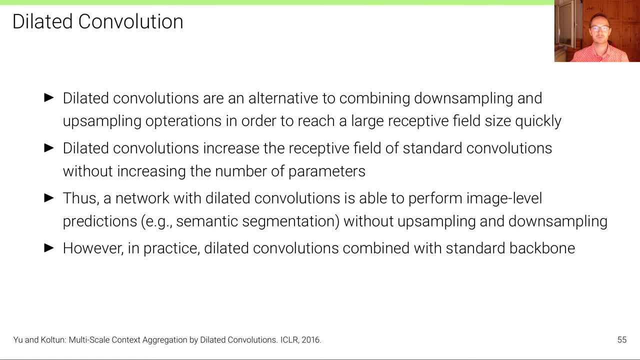 to this combined down and up sampling because they allow to reach a large receptive field size relatively quickly, just with convolutions. dilated convolutions increase the receptive field of standard convolutions without actually increasing the number of parameters. this is key- without increasing the number of parameters. 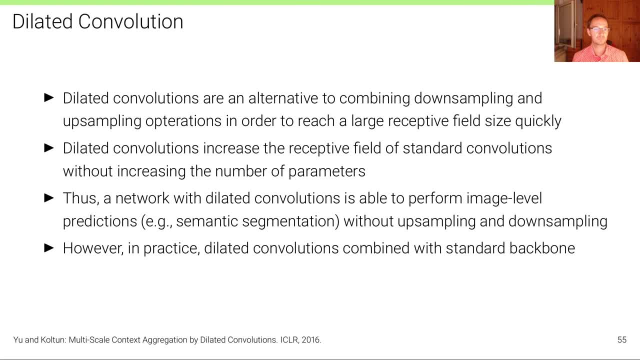 i can increase the kernel, the receptive field, and this is the core idea of dilated convolutions and therefore a network with dilated convolutions is able to perform image level predictions, for example in semantic segmentation, without upsampling and downsampling- in theory, in practice, now even in this work here, where this idea has. 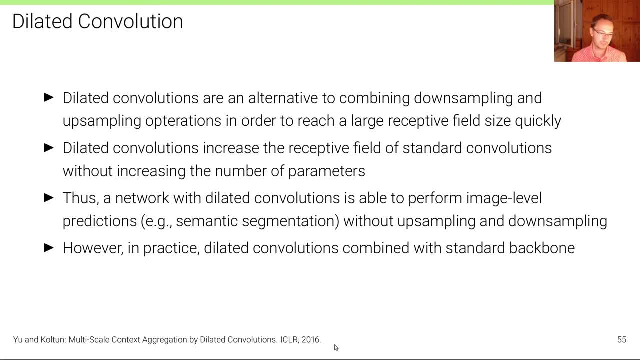 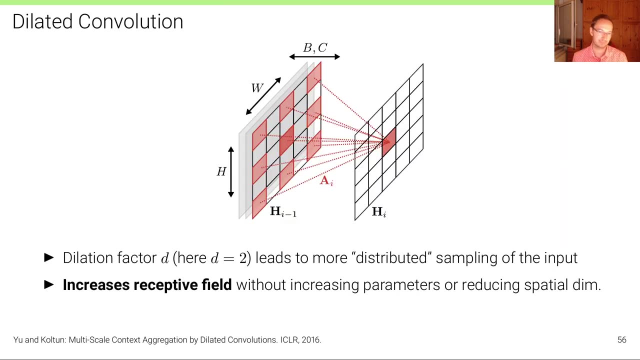 been presented has been presented concurrently in multiple works, so even in in this work here, for example, they still require a standard unit backbone and and could just do this on top to refine the segmentation, but then they could get much, much more details and much better quality. so let's look at the dilated convolution. how does the dilated convolution look like? well, 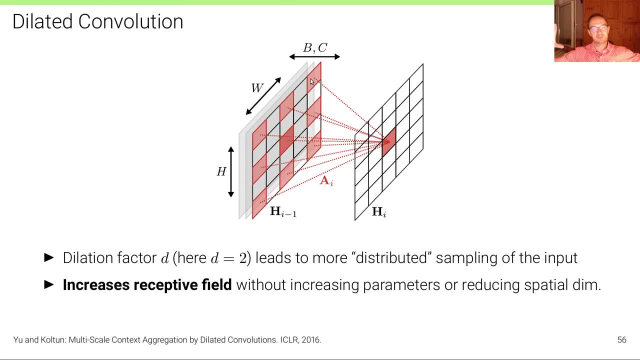 we have a dilation factor here. this is in this case. dilation factor is two and that distributes the sampling of the input signal. it's the previous layer, this is next layer, so we increase the receptive field size because we're effectively skipping some locations, so at the expense of 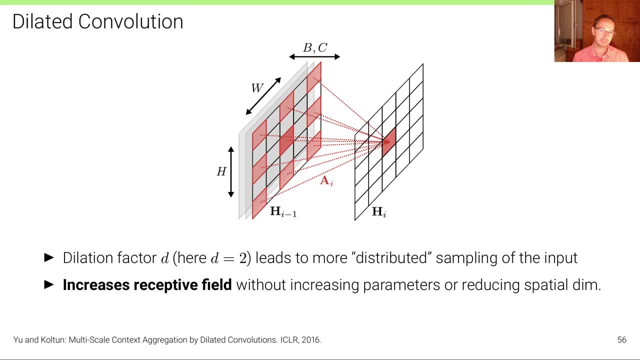 skipping some locations and potentially also introducing some, some artifacts, some mosaicing, some aliasing artifacts. we are increasing the receptive field, but we are not increasing the number of parameters. this kernel still has three by three times the number of channel parameters, no matter what the dilation factor is, and that's the crucial thing. 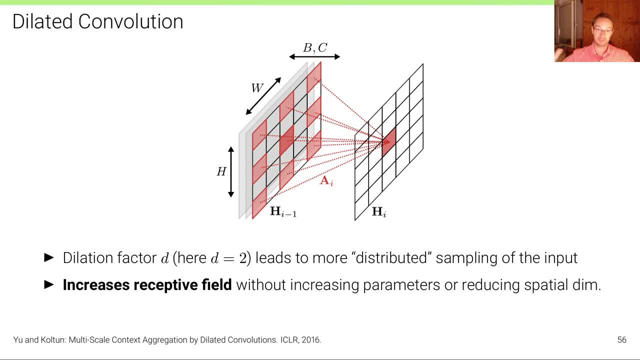 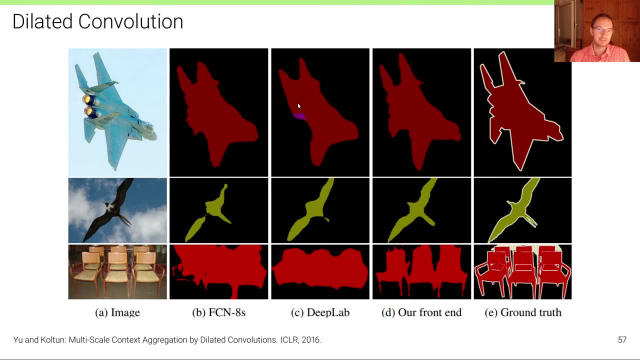 you can now use even higher dilation factors and get large receptive fields and combine this and here are some results. so you can see, this is the, the fcn, the basic version. uh, no, this is the fcn- uh, the fine version. this is the deep lab model and here is the. this is one of these state-of-the-art backbones combined with the. 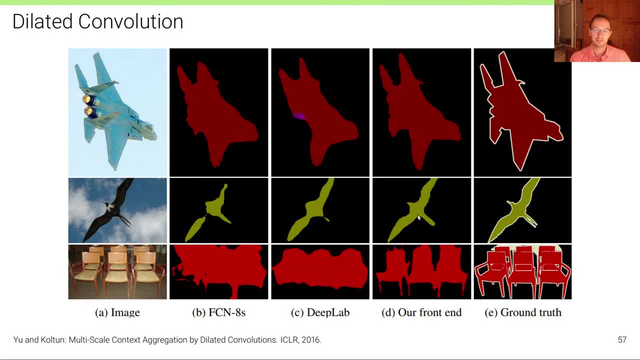 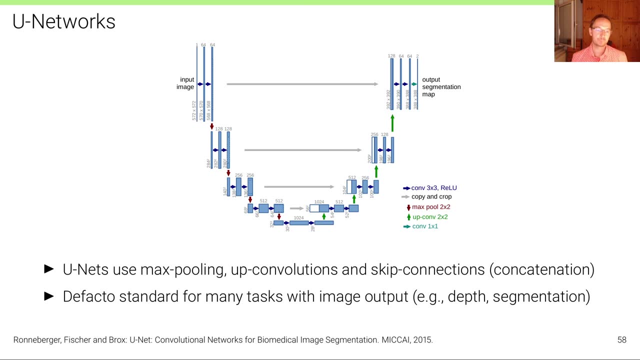 dilated convolution as the front end, you can see that this model achieves much higher accuracy. how much more detailed boundaries compared to these, these models. yeah, here's another model, also from 2015. it's called a? u network. very simple, very similar ideas, also one of the standard models. this is also has an encoder. it has a decoder, has. 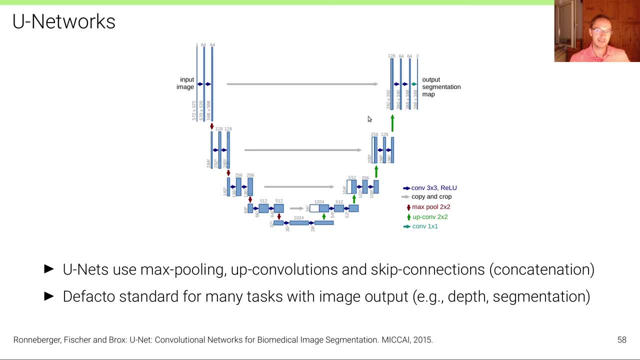 skip connections. but in this case, here the skip connections are concatenating the features from the respective from the same resolution, um, with the upsampling predictions from the previous resolution. in the decoder here the white and the blue. the white comes from the previous encoder layers at the same resolution and then 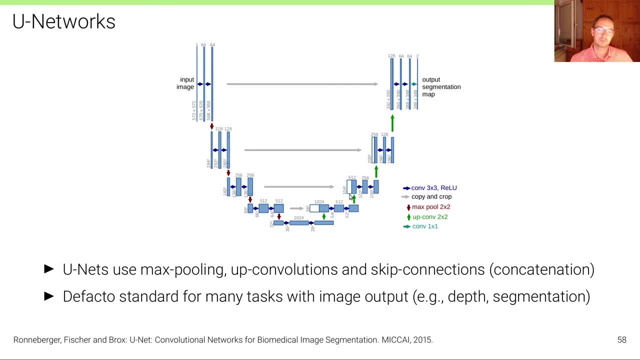 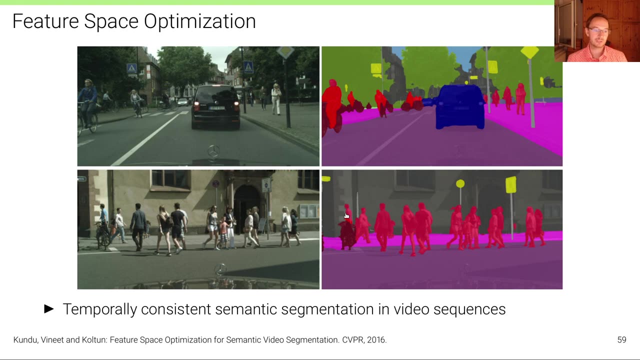 this is concatenated with the upsampled result of the decoder stage here, and this is one of the de facto standard architectures for many tasks with image level outputs, such as depth estimation or segmentation. here's a work where semantic segmentation has been tried to be made temporally consistent. if i apply a semantic 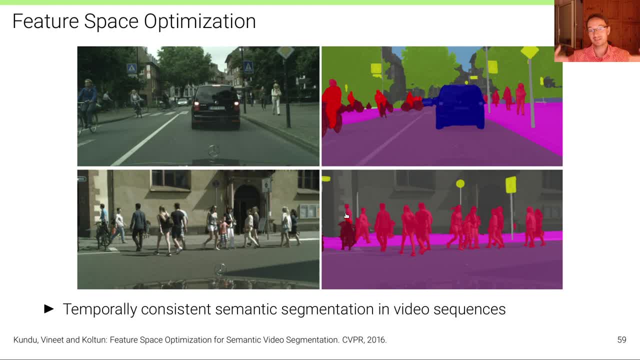 segmentation algorithm. it's not necessarily semantically temporarily consistent, because i apply it to each frame independently, and so there's a lot of flickering artifacts, a lot of noise going on, but here they optimized this model to be temporarily consistent as well, and the results even for this is 2016.. 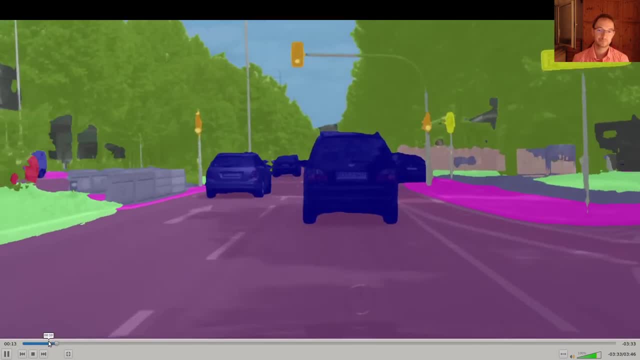 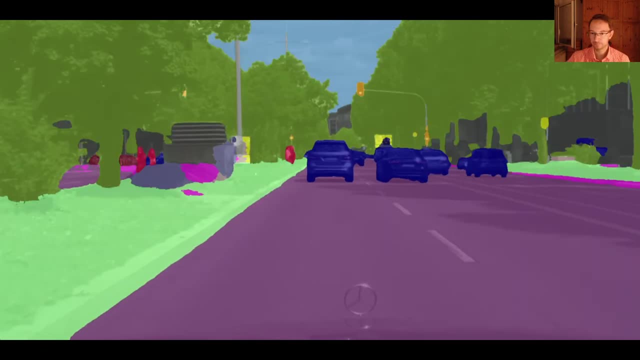 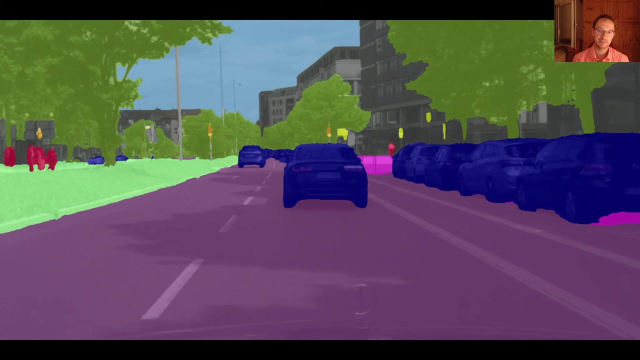 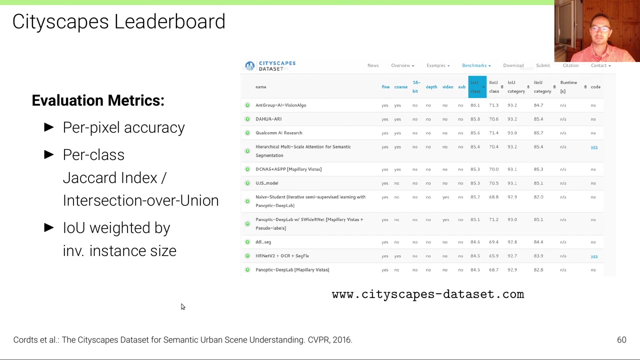 are really, really quite impressive, i think, so i let this play for 10 seconds. this is on the cityscapes dataset. here's the cityscapes leaderboard. this is one of the standard benchmarks for evan's evaluating semantic segmentation methods in the context of self-driving, and you can see: 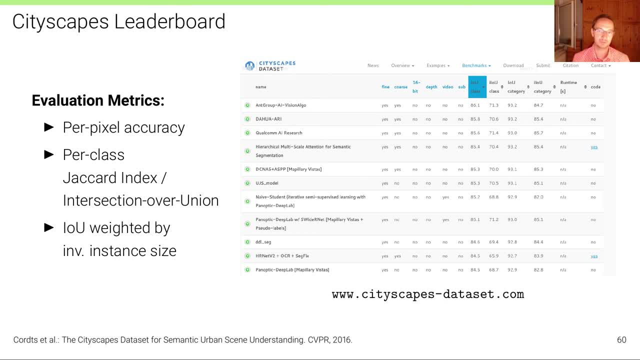 what is the state of the art? There's a lot of methods ranked on the leaderboard. You have to submit your results on a dataset, a test set for which the ground truth is not available, and the server evaluates your method, similar to the ImageNet challenge. 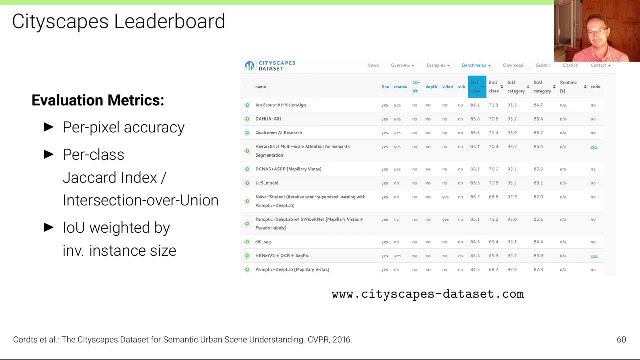 or the KIDI dataset, and then it creates a number and you can put your entry, your method, into that table. And the measures that are used for evaluation of semantic segmentation methods are. the simplest is per-pixel accuracy- just measure how many pixels are correct. but that's not used very. 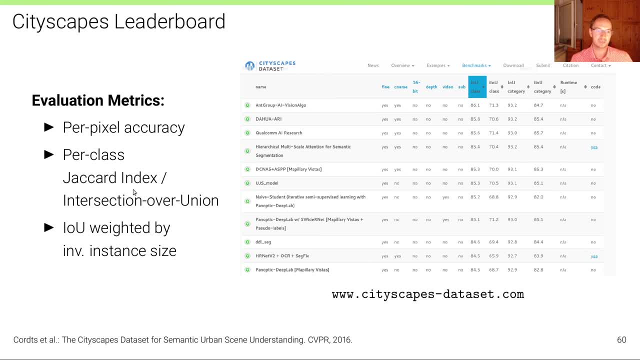 often More frequent these days, are per-class Chakar index or intersection over union. This is basically for each semantic class, We measure True positives and false positives and true negatives and false negatives in terms of, for that semantic class, comparing ground truth to the prediction. 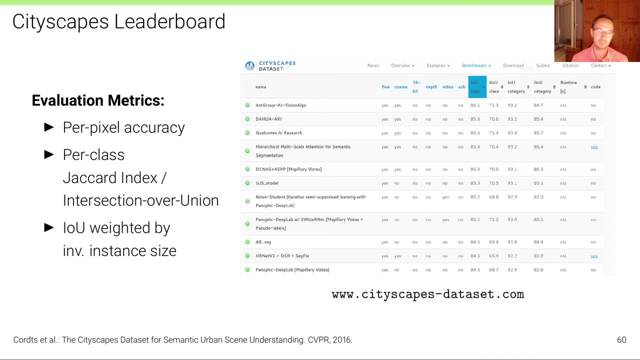 And this is also a metric that we'll talk about a little bit more in the detection unit later on. And then, because some of the semantic classes, due to the perspective projection and to the size of these classes, are very small By only a few pixels, there's also metrics that weight them relative to the instance. 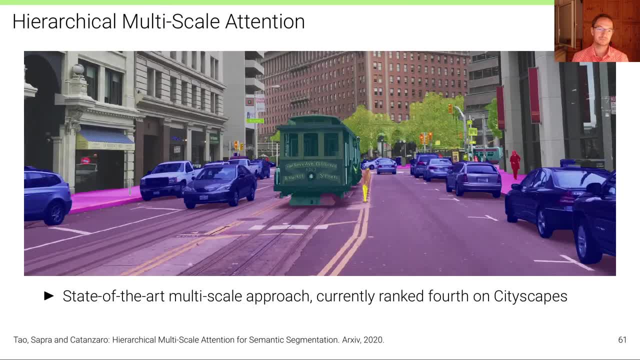 size- And here are results of a state of the art multi scale approach as of 2021, which is currently ranked fourth on Cityscapes, And you can appreciate all the details that are predicted by this model at really high resolution. You can see, for example, this pedestrian, these traffic lights here, these signs. 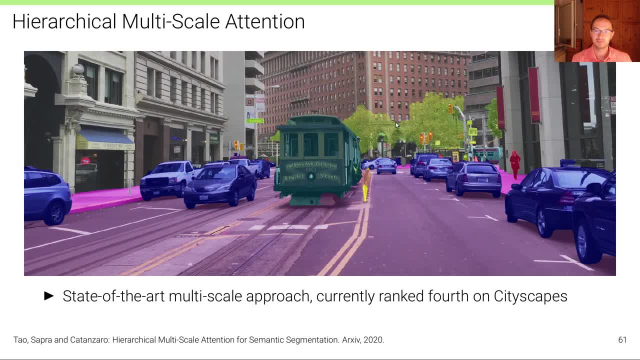 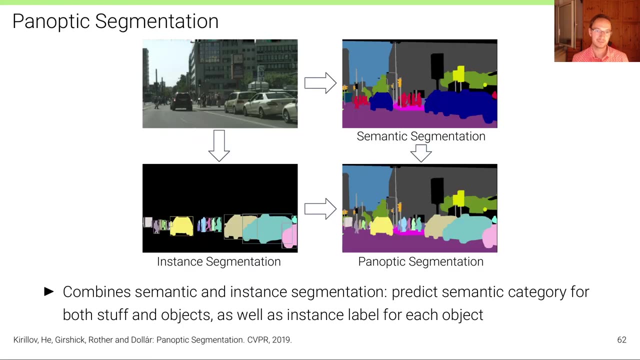 the boundaries, of the trees, of the buildings, of the cars, etc. It's really amazing what these deep neural networks for semantic segmentation are able to achieve these days. And what I mentioned already in the beginning: one task that is basically combining different you know, combining the semantic 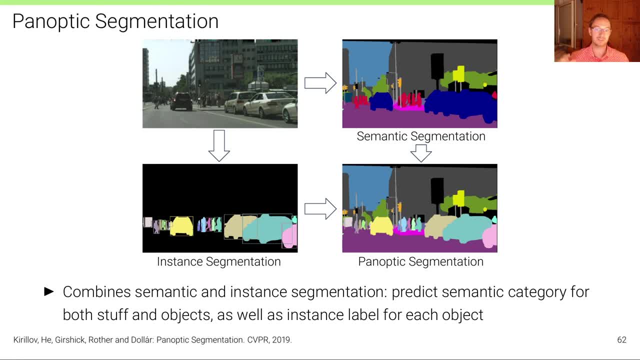 segmentation problem with the instance segmentation problem that we are going to discuss later in the lecture is called panoptic segmentation. So here the goal is to predict for each pixel the semantic category for both the stuff and the objects, as well as the instance label if there is an object. 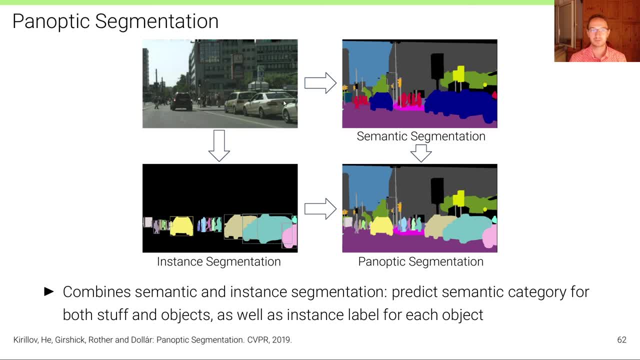 below this pixel. So this is called panoptic segmentation. Thank you very much.